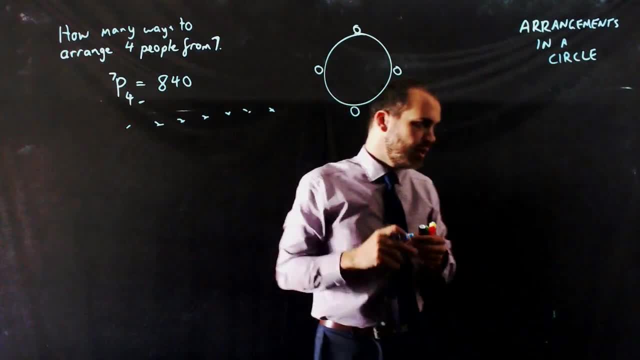 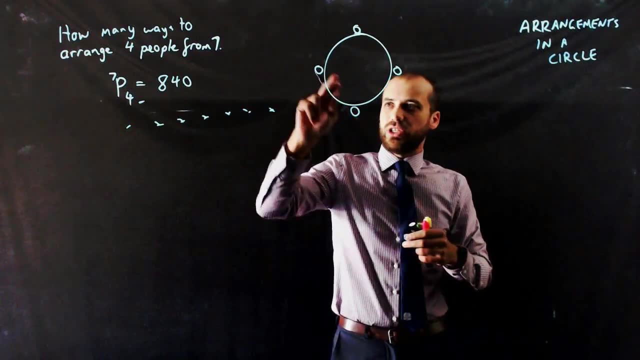 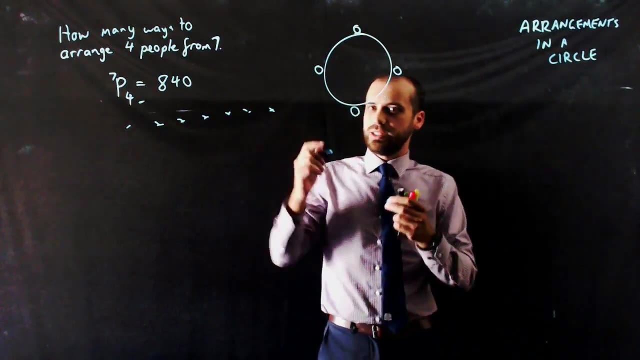 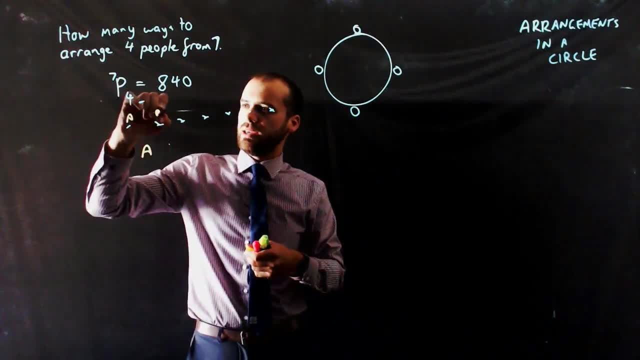 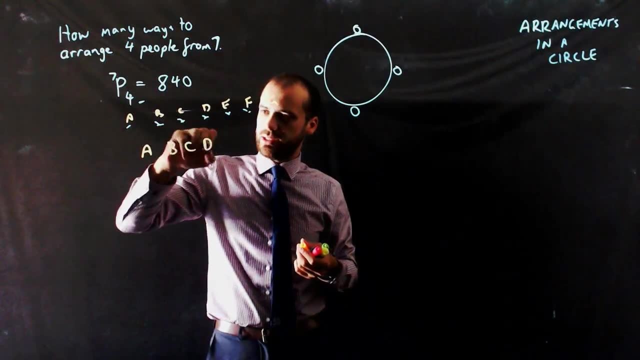 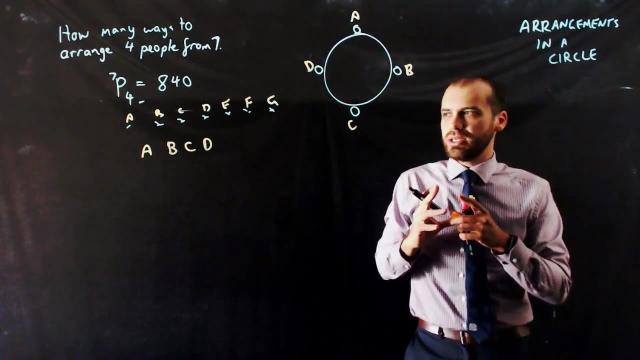 this arrangement here. So if I call these A, B, C, D, E, F, G, Now if I use the arrangement A, B C D and I seat them here like this, it should be clear that A, B C D is actually the same arrangement. 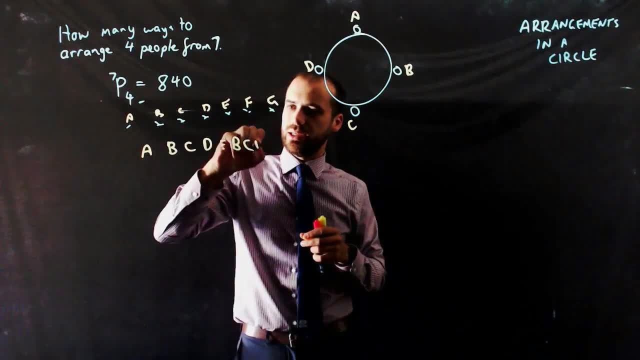 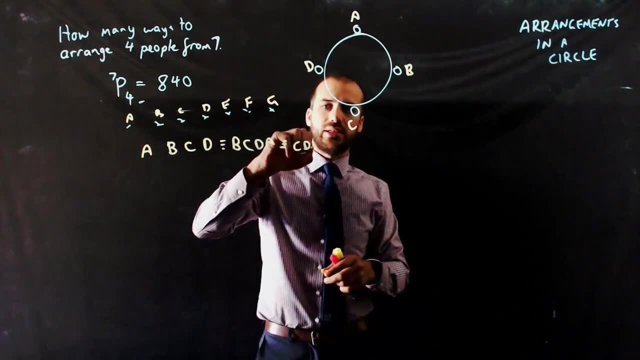 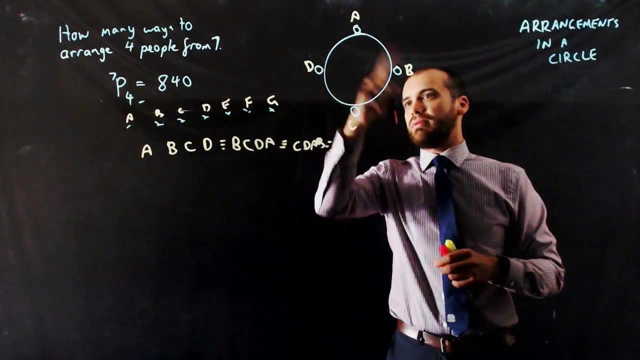 as B C D A, which is the same arrangement as B C D A, Same arrangement as C D A B, which is the same arrangement as. what am I missing? A, B, C D. 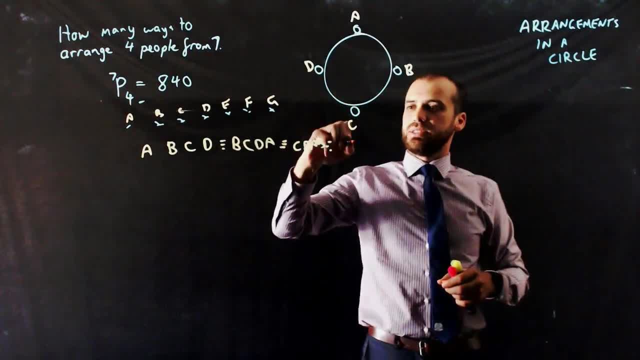 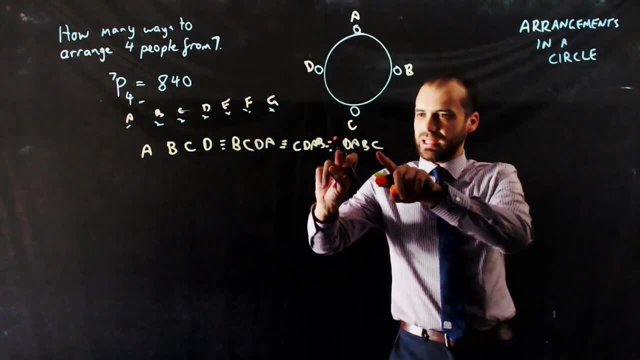 B, C, D, E, C, D, A, C, D, B, A. It's the same as D A, B, C, Because the same people are always sitting next to each other because of that link up. See C is sitting next to D, C is sitting next. 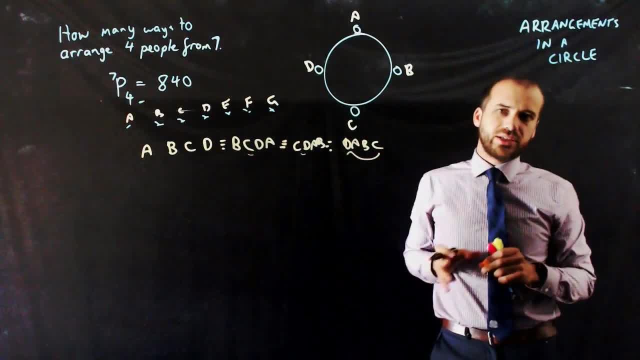 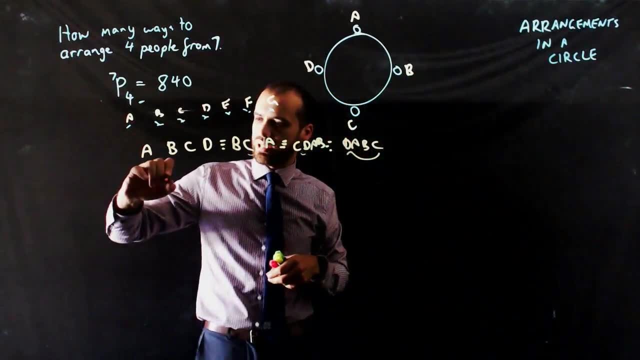 to D. here C is sitting next to D. here C is sitting next to D. here, Everyone's sitting next to the same people. Now, if you need to arrange something in a circle, the formula for that is going to be NPR over R. 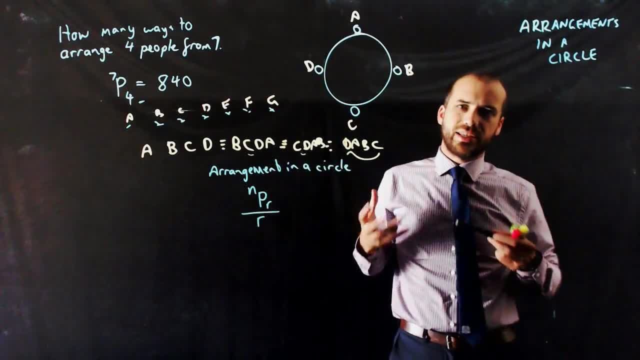 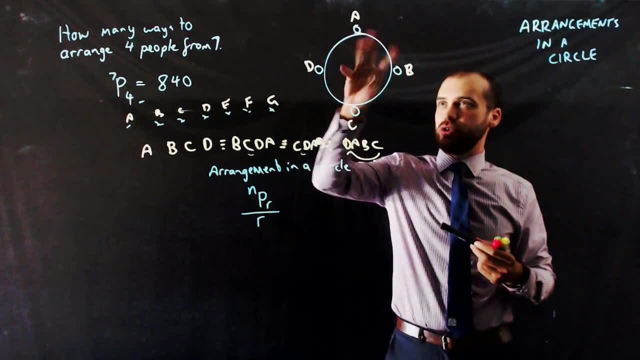 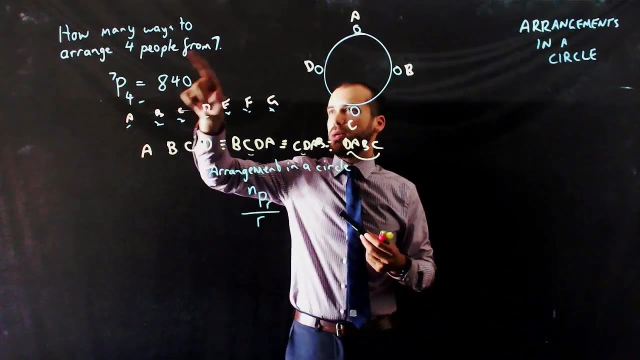 where R is the number of people that you're seating in that circle, or number of things that you're putting in that circle. The reason for that is because you rotate it through R times. In this case, we rotate it through four times. So how many ways to arrange four people from? 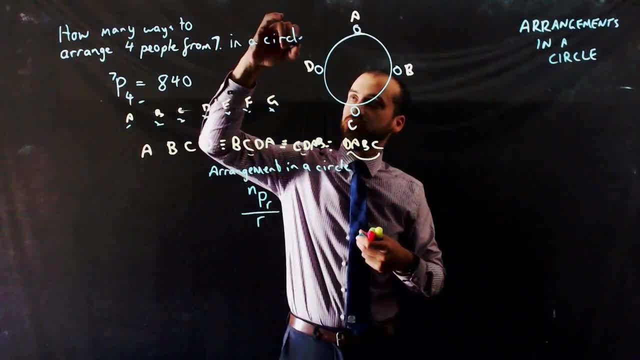 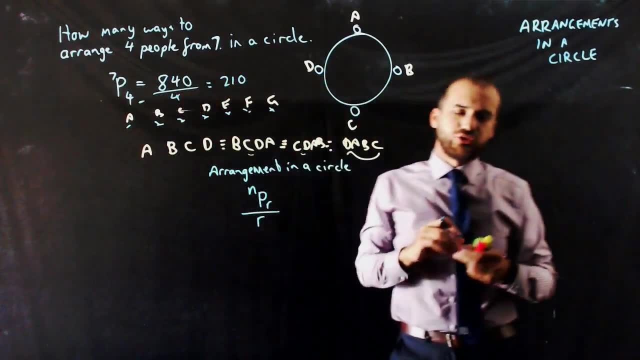 C. Well, the answer would be 840 divided by 4, which would be 210.. So drastically reduced just by putting them in a circle. All right, that's arrangements in a circle.